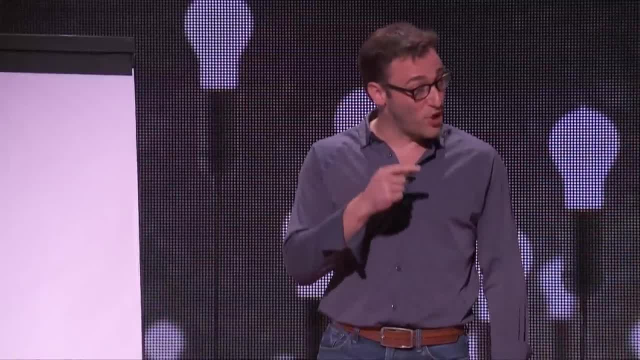 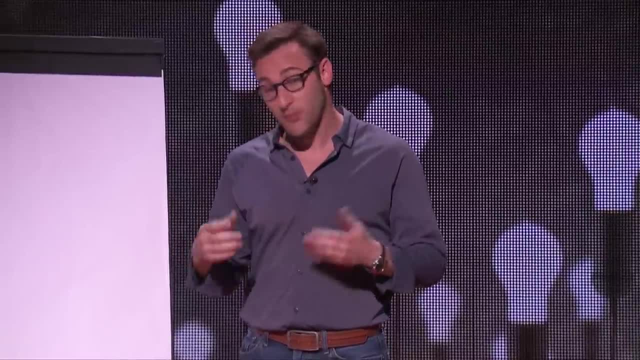 players, the rules are changeable and the objective is to perpetuate the game. When you pit a finite player versus a finite player, the system is stable. Baseball is stable. So is conventional war, for that matter. When you pit an infinite player versus an infinite, 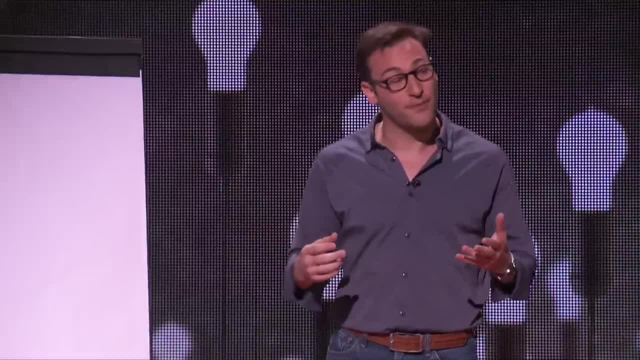 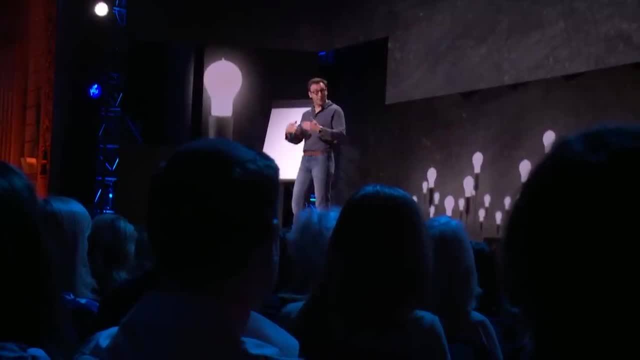 player. the system is also stable. The Cold War was stable- And that's because in an infinite game there are no winners and losers. We cannot lose the game, And so we work to keep the game in play right. In fact, because there are no winners and losers, the only thing a player can do is 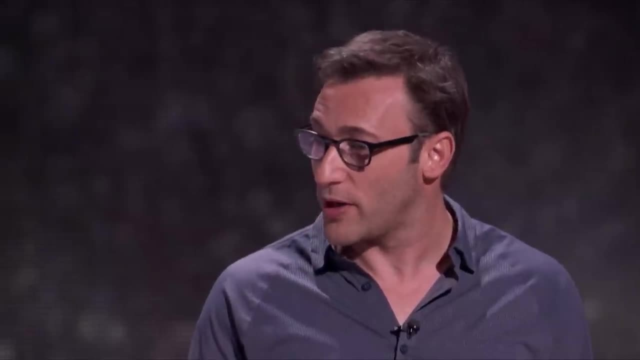 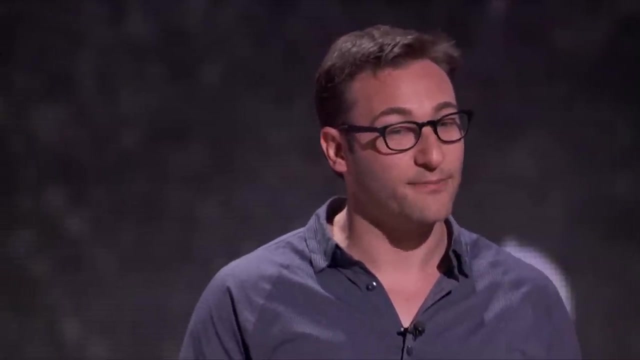 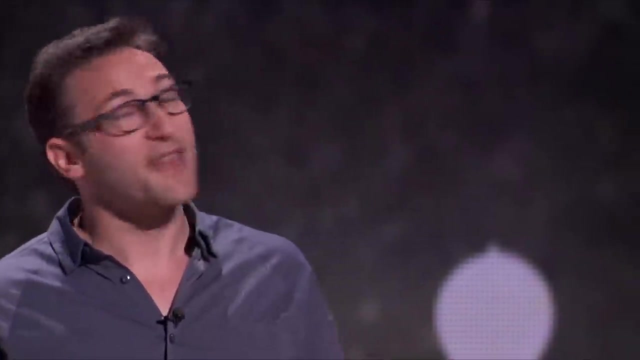 drop out when they either run out of the resources or the will to play. Problems arise, however, when you pit a finite player versus an infinite player. It's the finite player who then gets caught in quagmire. This happens in business all the time. The game of business is an infinite. 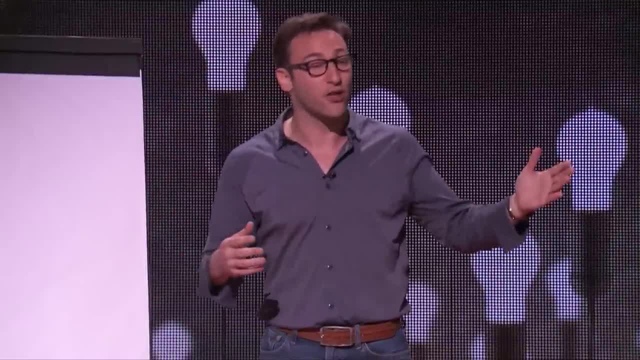 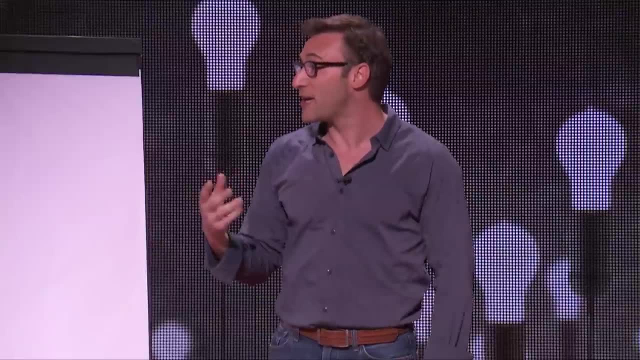 game. The concept of business has existed longer than every single company that exists right now, And it'll exist long after all the companies that exist right now go away. The funny thing about business is the number of companies that are playing finite. They're playing to. 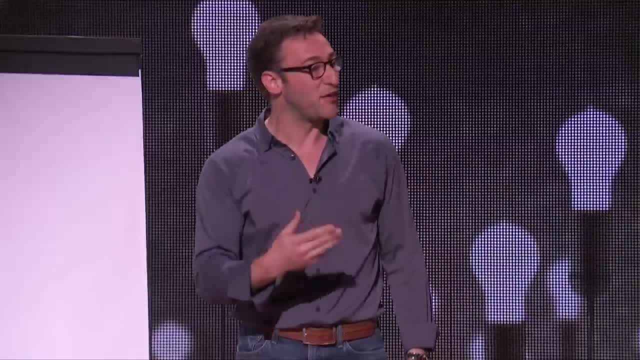 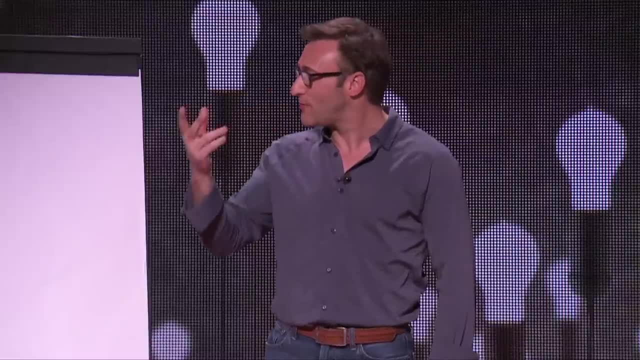 win. They're playing to be the best, They're playing to beat the quarter or the year And they're always frustrated by that company that has an amazing vision, a long-term vision that seems to drive them crazy And over the long term, that player will always win and 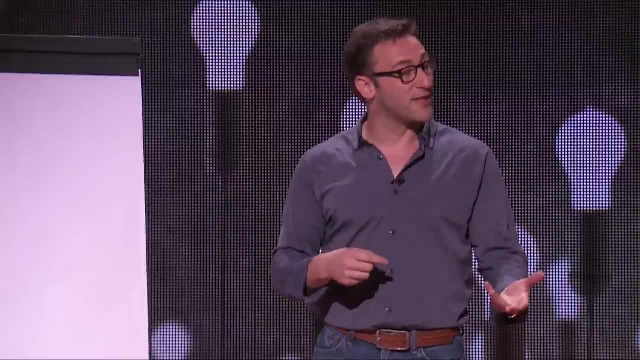 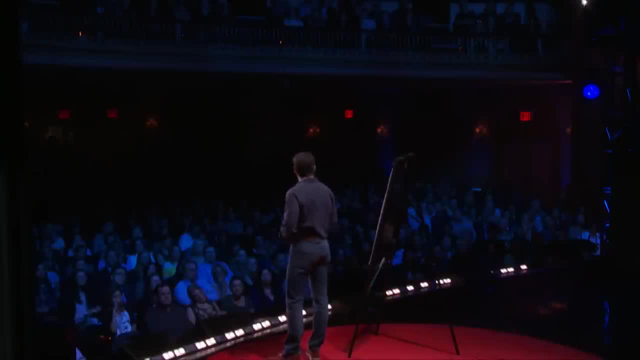 the other player will run out of resources or the will and they'll either go out of business or be banned. The way the game of business is set is always to win. You can't really say it's not best or best, because you're not winning on purpose. You're only winning in the hands of society. 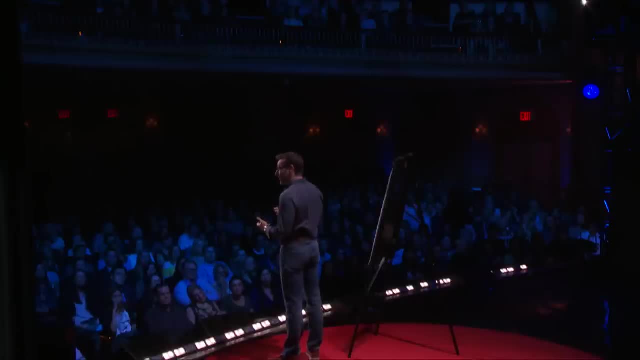 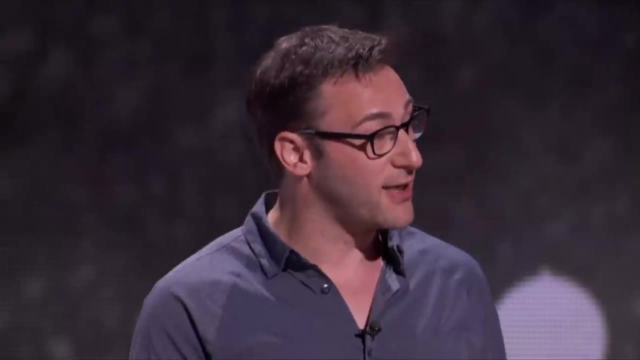 It's not being a organizer, It's a program, It's a mechanism, It's a mindset, It's a system. You have to be a political leader, You have to be the leader in the whole of the country When our economy has collapsed. it's not a political game, It's a political game And 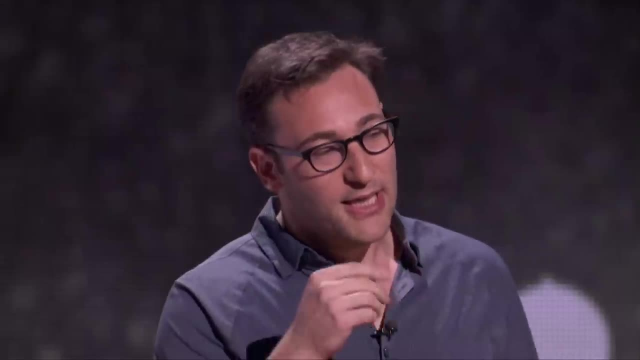 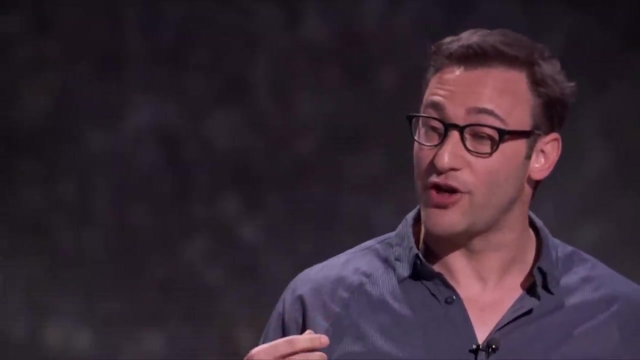 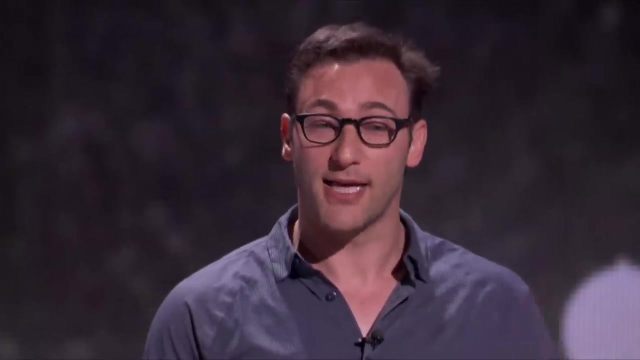 it's really a political game, And this became completely clear to me when the Soviets actually drove their tanks into Afghanistan and Brzezinski. the National Security Advisor for President Carter was called into the President's office and the President asked him: what is the policy of the United States? 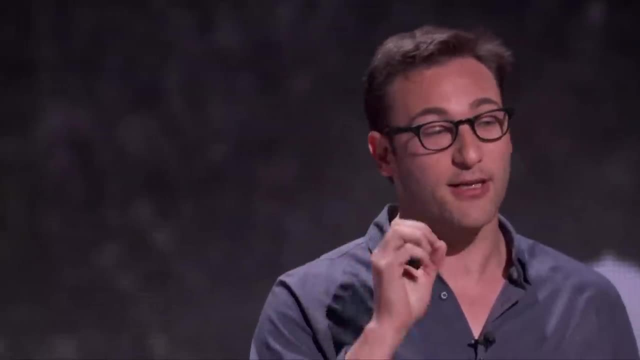 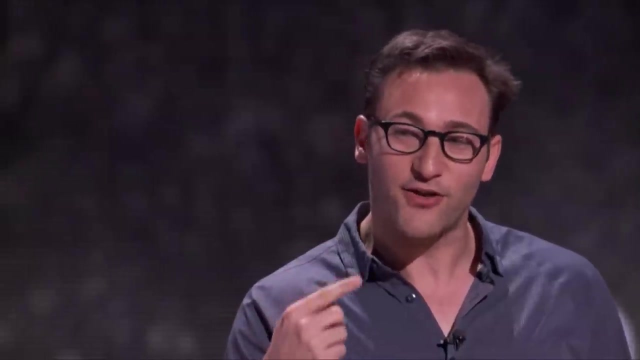 And Brzezinski said the policy of the United States is to eject the Soviet. It's a finite goal. And then, almost as an offhanded comment, he says: and if we can't do that, we'll make it as expensive as possible for them to stay. 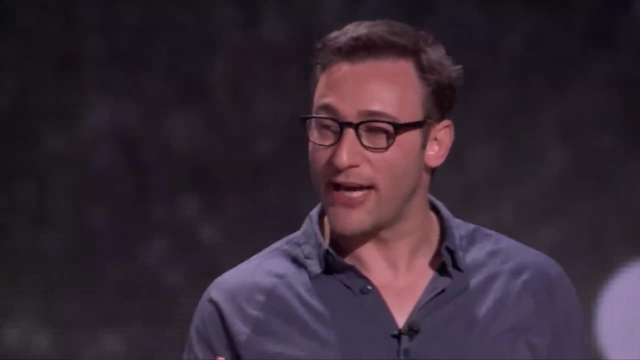 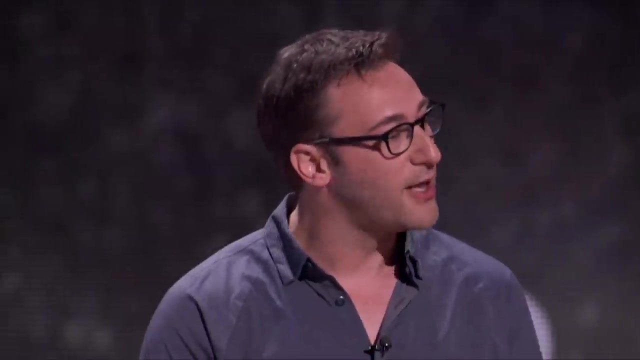 In other words, the United States accidentally had an infinite strategy which is not fixed in time and we don't know exactly what it looks like. What we're trying to do is drain the enemy of will and the resources to continue to play. 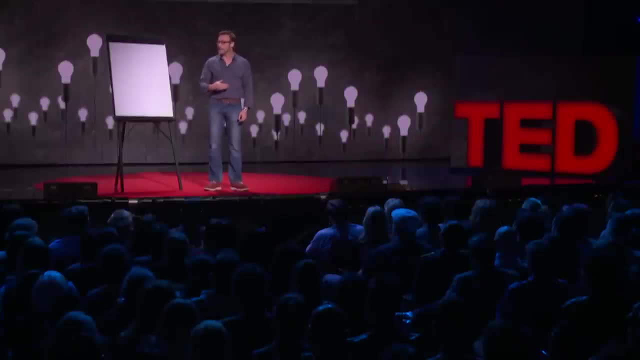 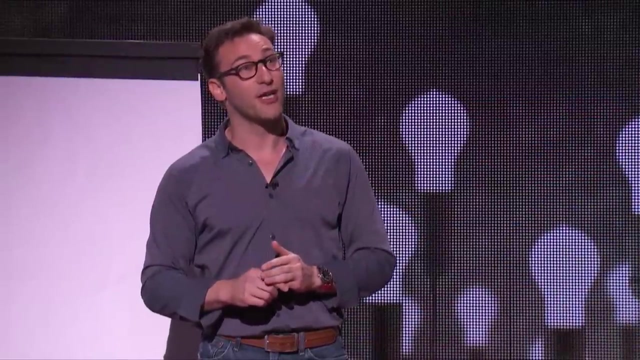 And ten years later, the Soviets drove their tanks out of Afghanistan, running out of resources and the will. Now, if you think about what happened when the Berlin Wall came down, we were in an infinite game- Soviets and the United States- and the Berlin Wall came down and the United States made again one of the greatest, perhaps one of the greatest blunders- policy blunders of the 20th century. 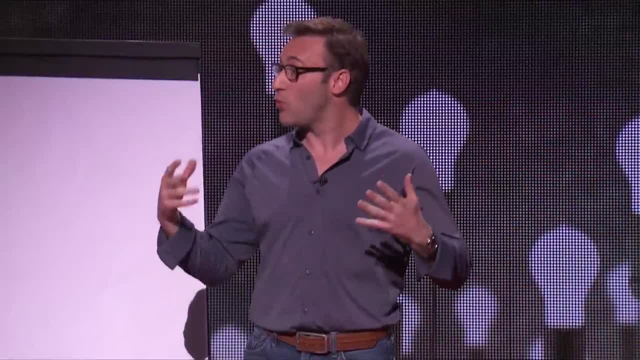 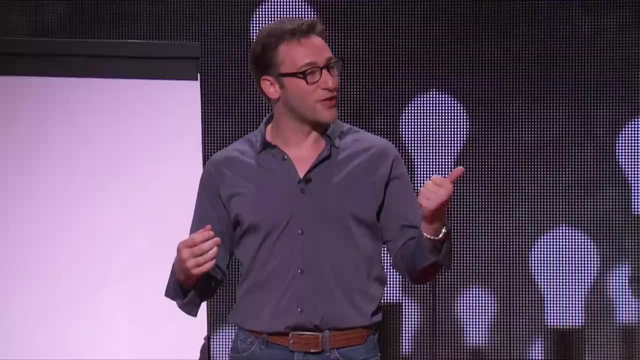 They announced that they had won the game. They had won the Cold War. No, they didn't. The player dropped out because they ran out of the will or the resources to play, And the problem is is that they didn't have the resources to play. Because they thought they had won the war, they started acting like victors And the United States imposed their will on the world for about 11 years and, as it turns out, the world didn't like that too much And, as what happens in all infinite contests, new players started to emerge. If you consider how the Cold War existed, it really existed on three tensions. There was a nuclear tension. Both states had nuclear weapons to end all life. There was an ideological tension. One was an exporter of democracy and capitalism, the other one was an exporter of Soviet-style communism. 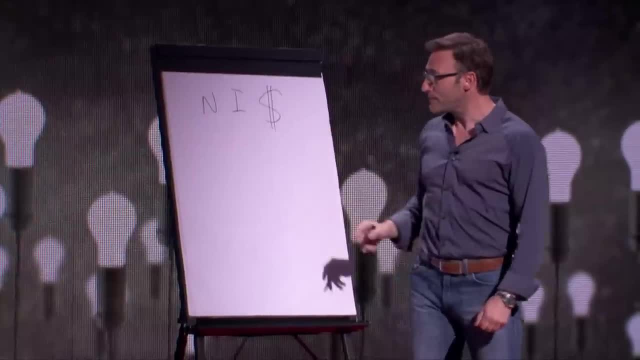 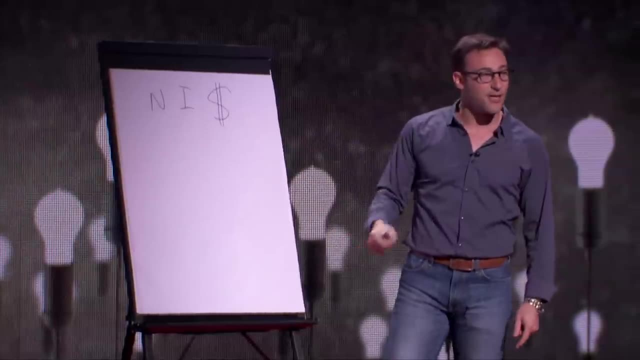 And there was an economic tension. That's what kept the Cold War alive and well, Not coincidentally. life, liberty and the pursuit of happiness: the only three things for which we will bear any burden and pay any price and fight forever to defend. Now the nuclear tension has been replaced by Pakistan and Iran and China. oh no, China was already there. Pakistan, North Korea, maybe Iran? the ideological tension, Soviet-style communism has been replaced by Islamic extremism and the economic tension. 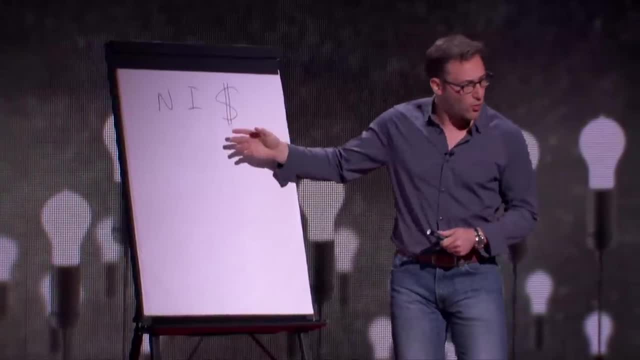 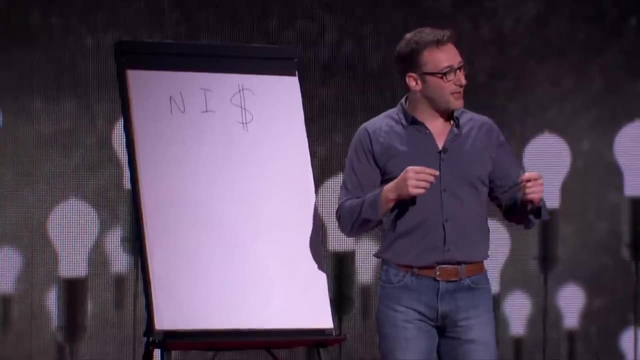 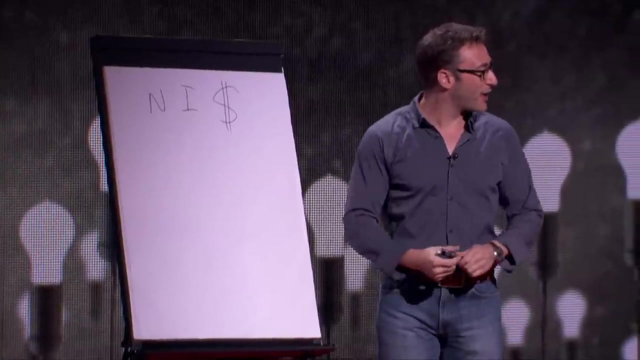 the Soviet Union's been replaced by China. We don't fear nuclear war with China, but the point is, all three tensions are alive and well And you see, the problem is they all know who their enemy is, but we don't realize that the Cold War 2.0 is happening And we are still trying to decide. 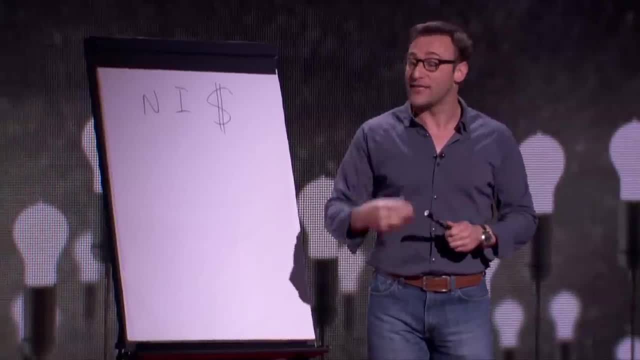 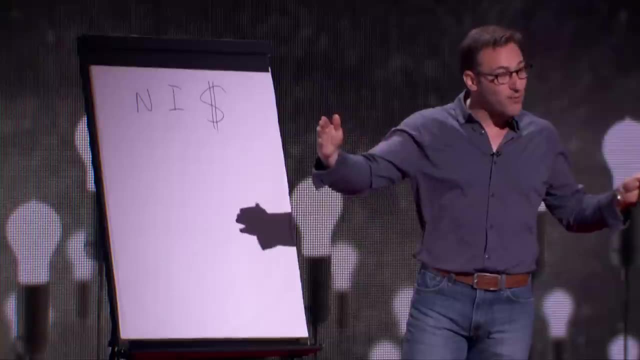 which one is more important. We're trying to win and beat all of these things and not realize that the game is infinite, not finite, And the United States policies these days have become shorter and shorter term, which creates turmoil and chaos in strategy and how we present ourselves. 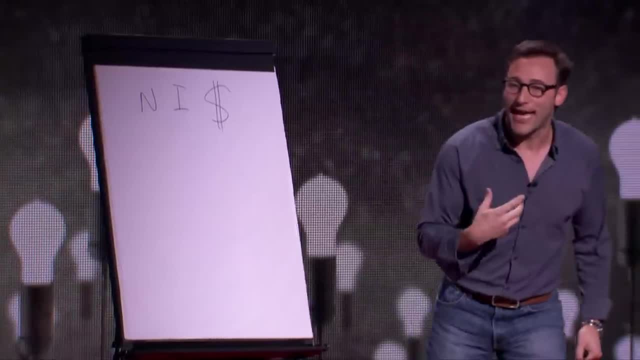 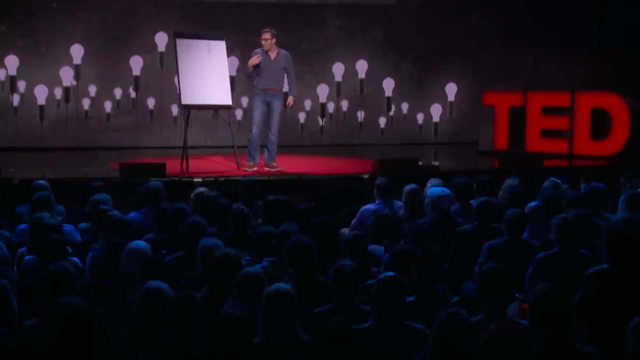 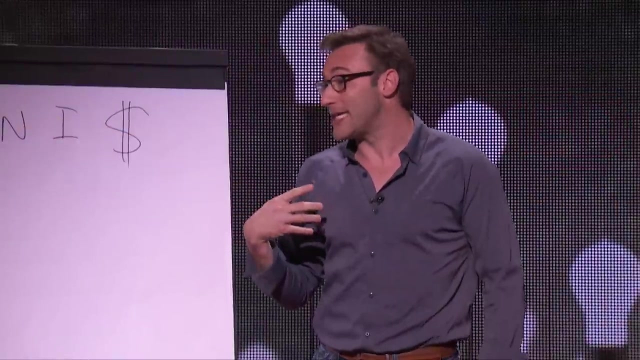 to the world. The easiest way to understand the game you're in is when you have an opposing force. In other words, not that right. So you want great leadership. You want somebody to say what we stand for, but if you don't have that, you get to say not that. So it was really easy. The intelligence services, for example. during the Cold War they fought like cats and dogs, like they fight now, but they could all agree on one thing: not that. And they worked really, really well to combine their forces to face the Soviet Union. We don't have a singular not that anymore, and so 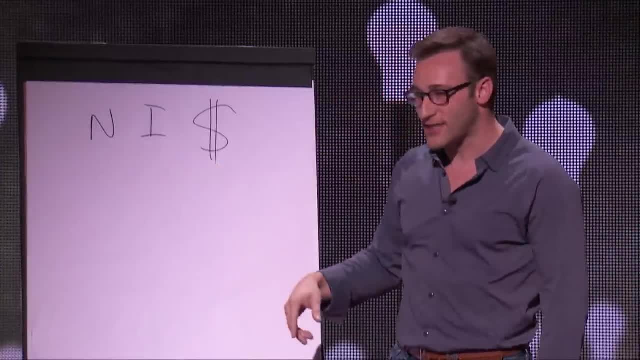 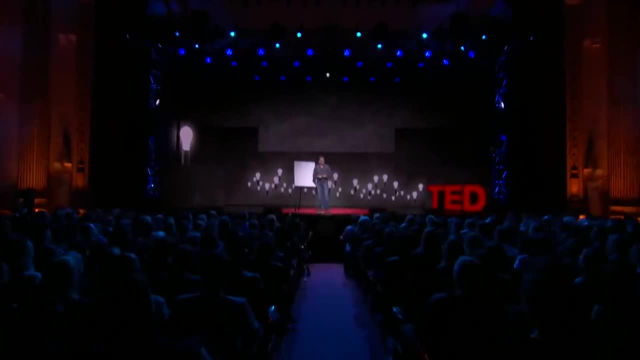 we're all over the place, But all of our enemies all have a singular not that. And it's us Ideally. we want to run all of our decisions through our values. These are what make us enduring. Our values are enduring, and this is what is the foundation of an infinite contest. 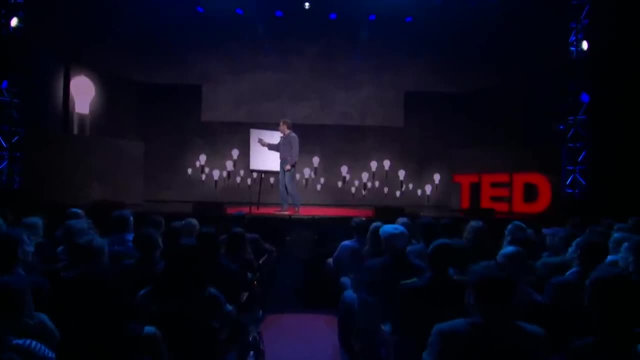 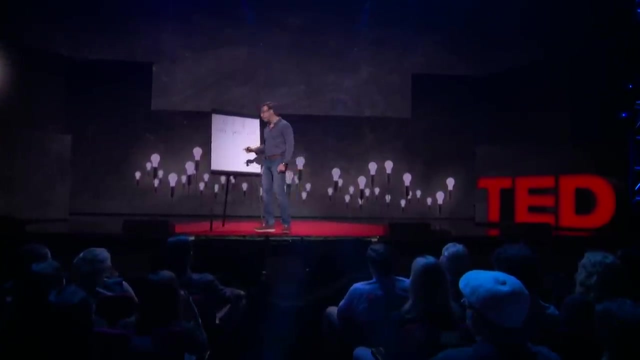 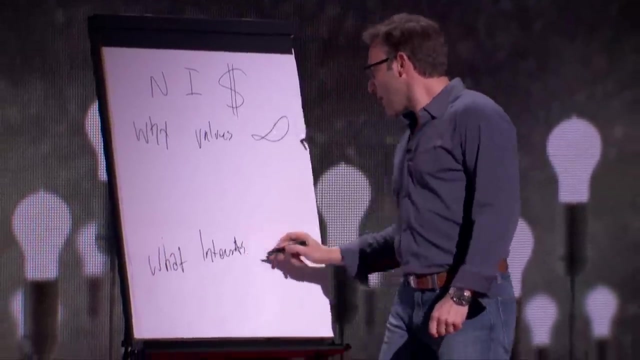 So you consider, up here is where our values lie, what I call the. why our values? right, These things are infinite. They're enduring. right Down here you have what I call the what. These are our values, and they are finite And ideally, what you want to do is you run all decisions through our 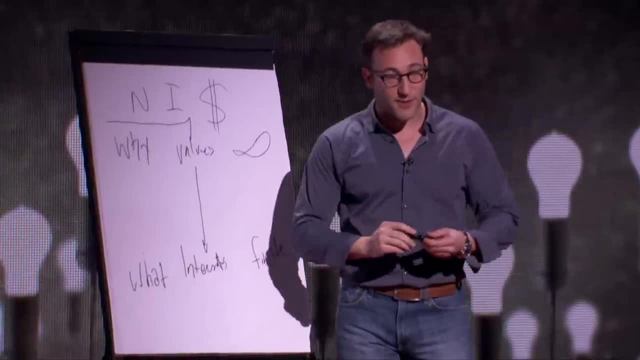 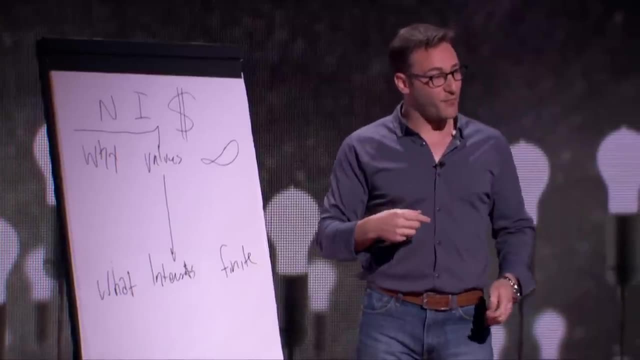 values and then through our interests. Let me show you what that looks like. Sometimes they go in our favor and sometimes they don't. So, for example, when we go into a battlefield and we shoot a bad guy, we will take his injured body, we will bring him into our hospitals and we will risk American 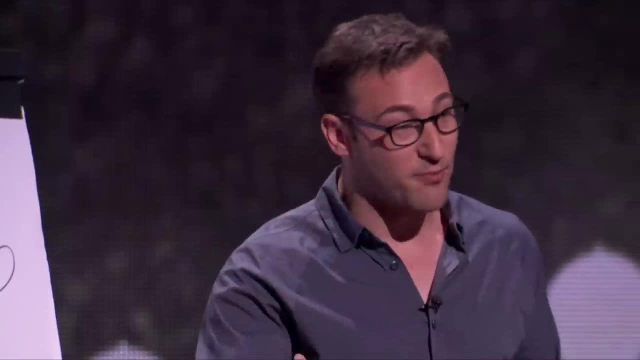 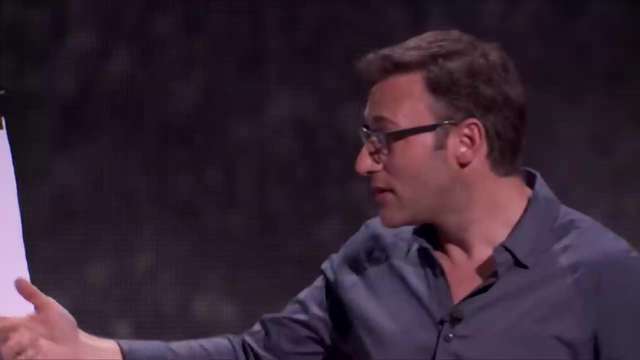 lives to bring him into the hospitals, use American doctors, American beds, American medicines to nurse him back to health. That's not in our interest. That's not in our interest. That's not in our interests. But the reason we do it, because it's kind of who we are, It's kind of what we do. It's. 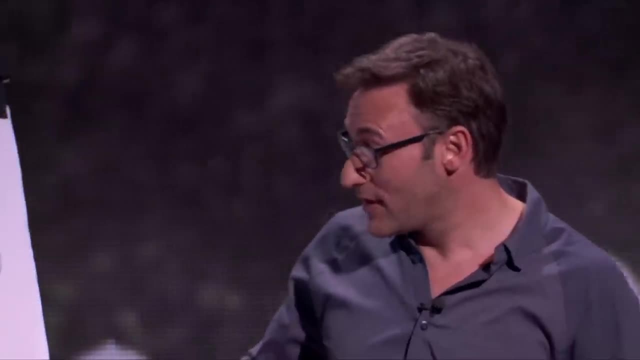 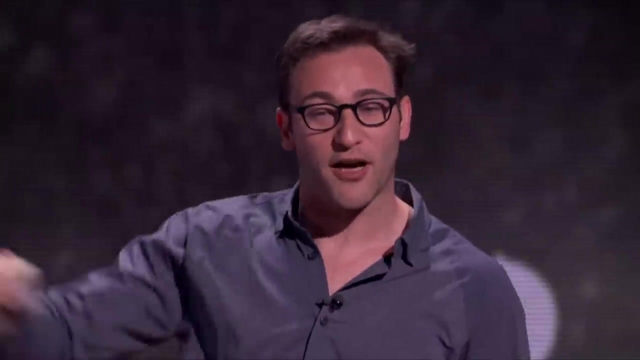 like it's our thing, right When we make a decision based solely on our interests. it looks like this right, So should we torture people? Now, the reason we did it offshore is because everybody kind of knew that that wasn't our thing, because if we had no problem with it, we'd just do. 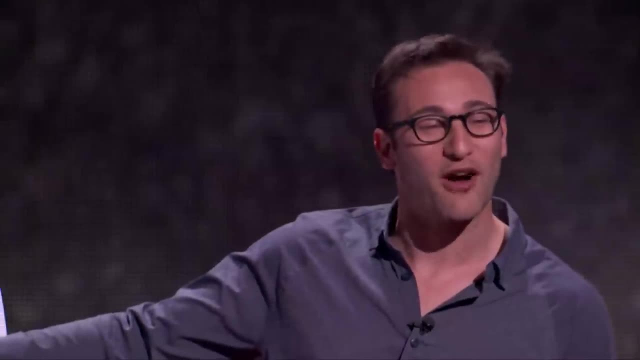 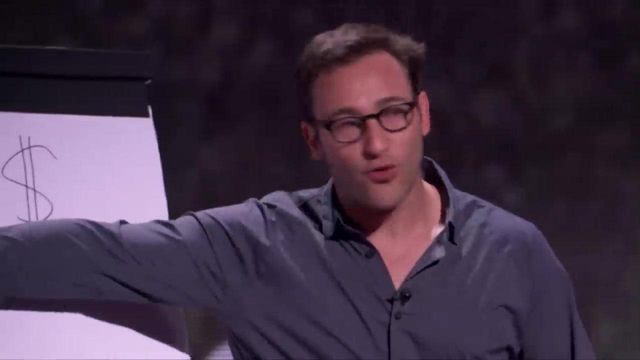 it here. So we hid it away because we knew it was uncomfortable, because we know what our values are. So what's been happening in the world is we've been evaluating all of the things that have been going on by ignoring our values, because we don't realize. 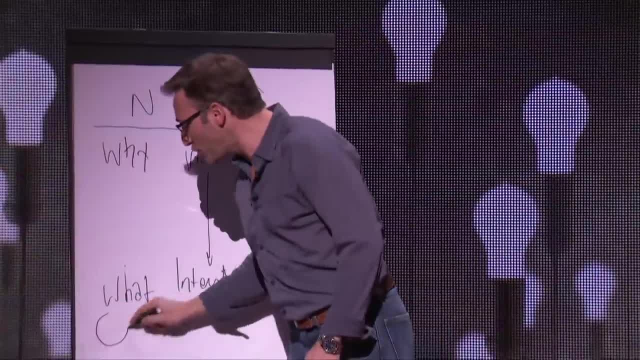 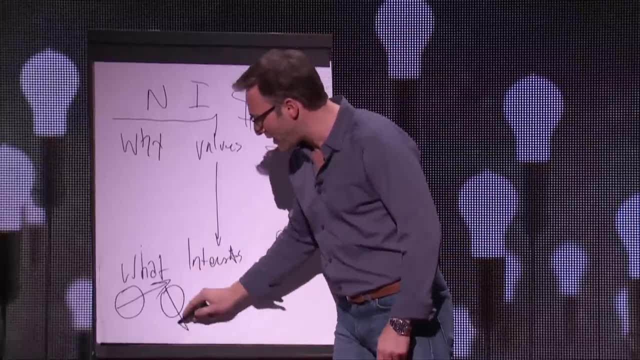 we're in an infinite contest and we only look at our interests. So we think about what should we do in Syria And we make a very, very good decision based on Syria, our interest in Syria, and we make a decision. And what should we do in Crimea, And what should we do with regards to Putin And what